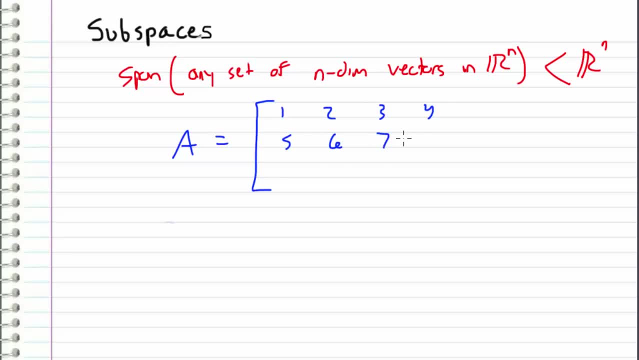 1,, 2,, 3,, 4,, 5,, 6,, 7,, 8,, 9,, 10,, 11, 12.. So we have this matrix. Then we can define subspaces that are associated with that matrix. 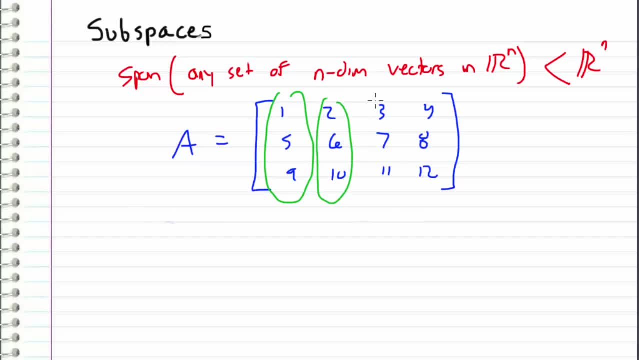 with this matrix by taking the span of the vectors that form the columns of this matrix. So if we call these V1,, V2, V3, and V4, and we take the span of this vector set, then this forms a subspace that we've referred. 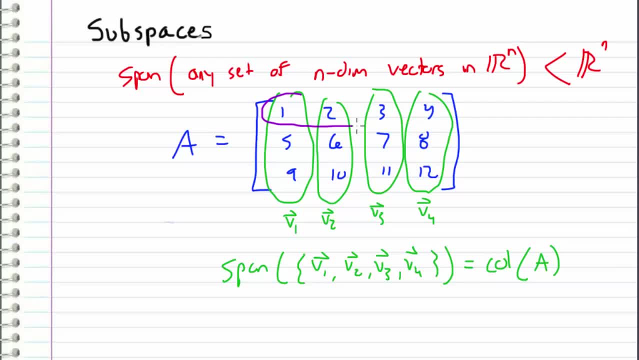 to the column space of A, And similarly we can take the span of the rows. And if we were to take the span of these rows, what we get is the row space of A. So the span of the vectors that form matrices creates subspaces that we are interested in. 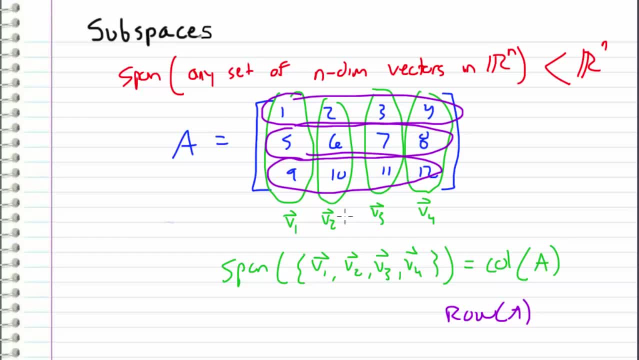 and we will be studying those later on in the series. So that's the reason why I wanted to point out that the span of any given vector set in Rn is a subset of Rn. So in this particular example, the column space. 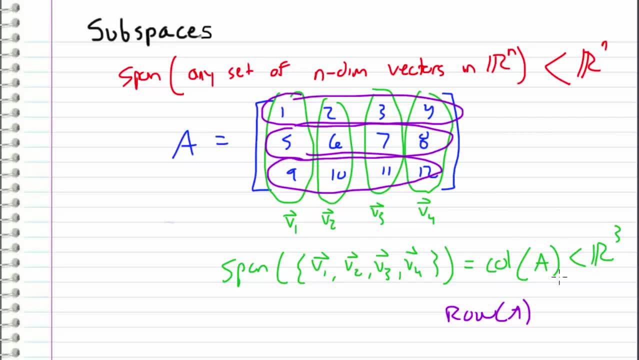 the row space of A is a subset of R3 because the columns, the vectors that form the columns, are three-dimensional. therefore they exist in R3.. And similarly, the row space of A is made up of four-dimensional vectors, so we can say that the row space is a subspace of R4.. 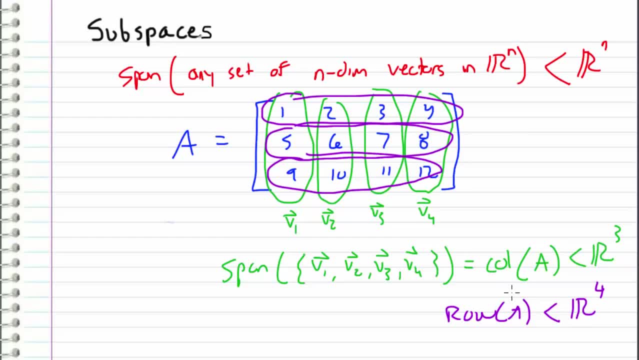 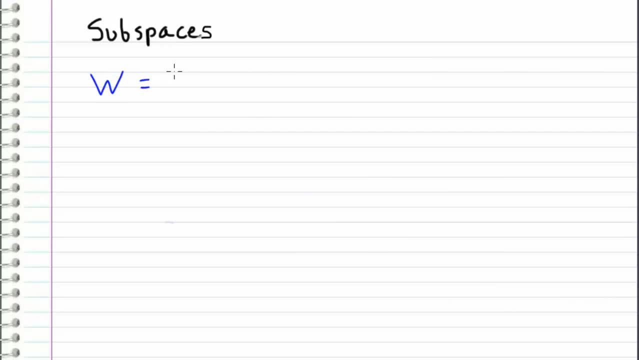 So, anyway, in this video I want to consider a specific example and determine whether or not it is a subspace or not. So let's define a set that we will call W, and let's say it is equal to the set of all vectors. 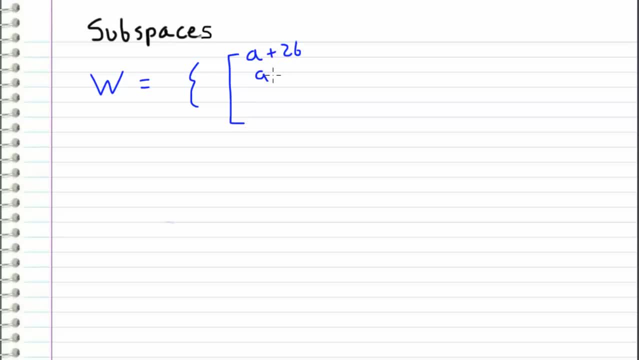 of the form A plus 2B, A minus B and 3B, where A and B are real numbers. So this space W or this set W contains all the vectors of this form for any A and B, and we want to determine whether or not W is a subset of R3,. 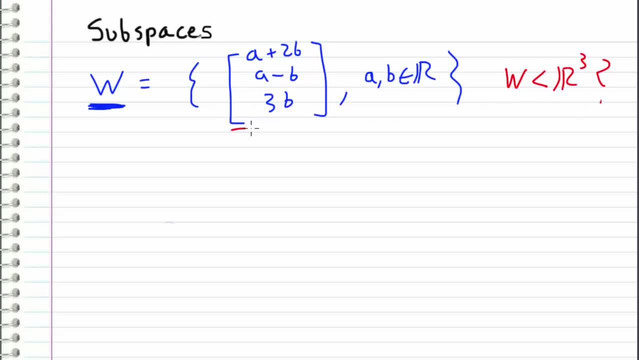 where R3 is the vector space that this vector lives in, because it is three-dimensional. So recall from the previous video: in order to determine whether or not something is a subspace, it needs to satisfy the three rules that we talked about. 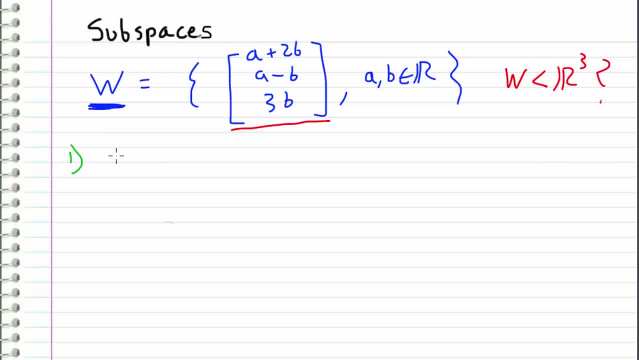 So the first one is that it must contain the origin. So if we let A equals B, which all equals zero, so if we set A and B equal to zero, what we get is the vector zero plus two times zero and zero minus zero and three times zero. 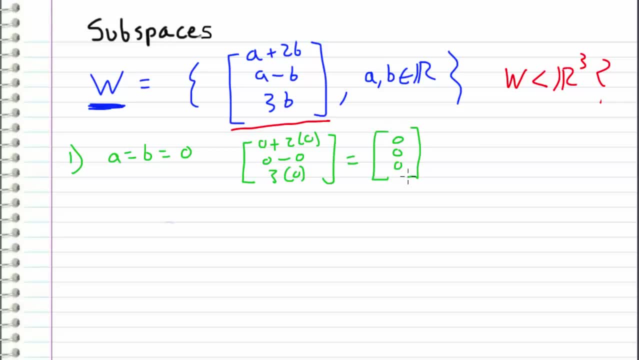 which comes out to the zero vector: Zero, zero, zero. So we know that W contains the zero vector. so we can say that this vector is an element of W for A and B equal to zero. So the second thing we want to check: 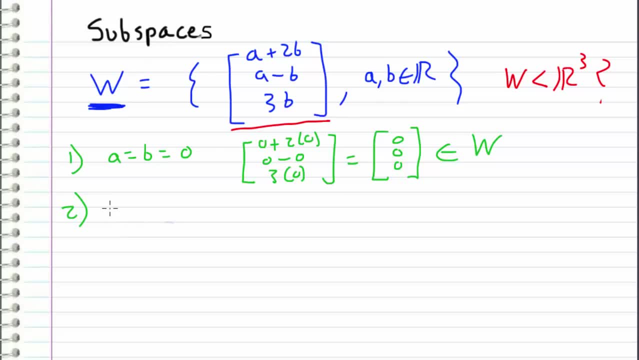 is whether or not this is closed under addition. So let's create an arbitrary vector W1, and let's let it equal A1 plus 2B1,, A1 minus B1, and 3B1, and let's pick another arbitrary vector, W1, and let's pick another arbitrary vector, W1,. 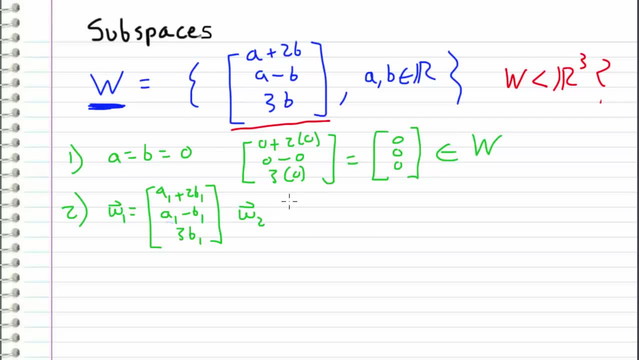 and let's pick another arbitrary vector, W1, in our subspace, and let's let it equal A2 plus 2B2,, A2 minus B2, and 3B2.. So recall that, in order to check whether or not, 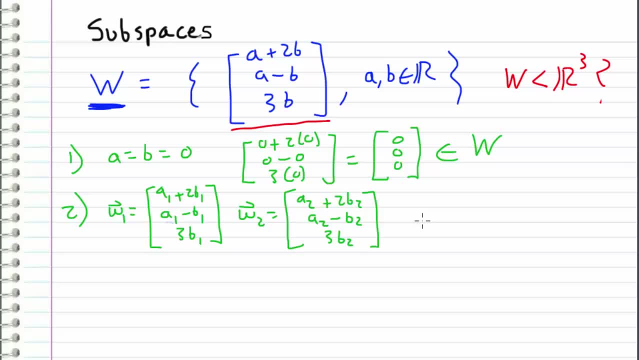 this is closed. under addition, we add them together and see if the sum is also in the subspace. So if we add these two vectors together- W1 plus W2, this comes out to be A1 plus W2.. This comes out to be A1 plus W2.. 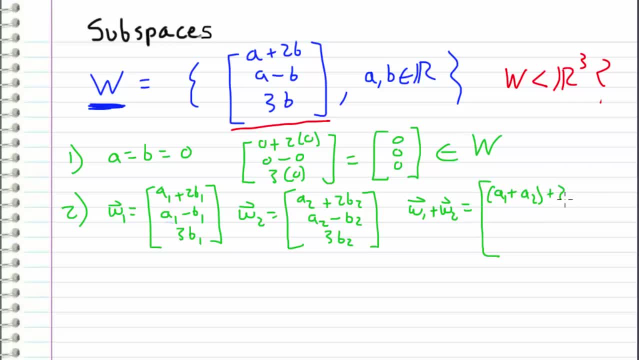 This comes out to be A2 plus 2 times B1 plus B2.. And then in the next entry we get A1 plus A2 minus B1 plus B2.. And then we get in the last row 3 times B1 plus B2.. 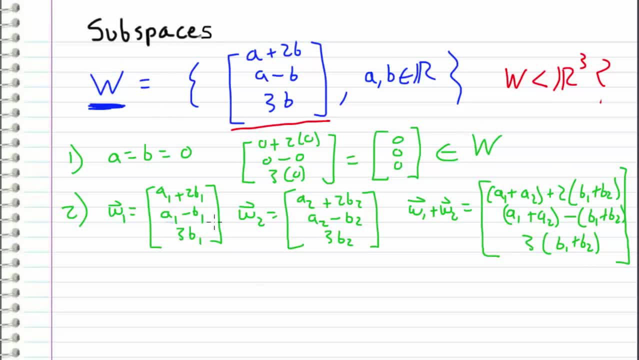 So, in order to check whether or not this sum is an element of W, all we have to do is see if this vector right here fits the form defined in our set, And upon inspection we can say: hey, let's let A equal to A1 plus A2,. 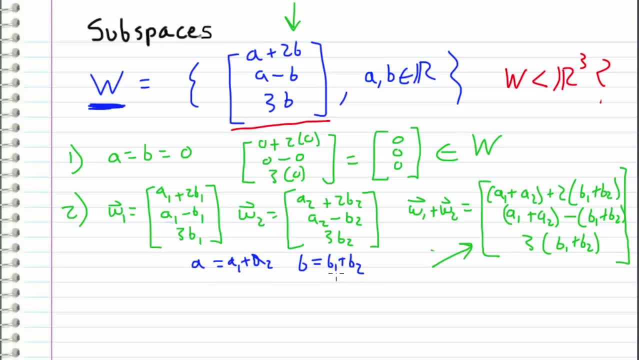 and let's let B equal B1 plus B2.. So if we were to replace, if we were to substitute in these expressions into our sum, what we would get is the vector A plus 2B, A minus B and 3B.